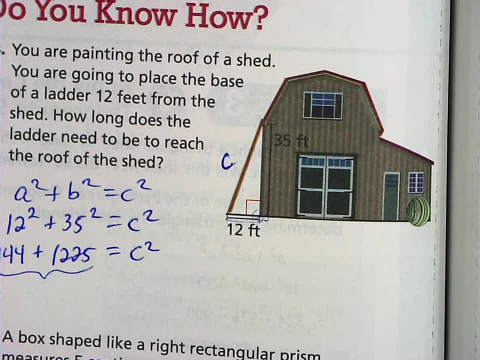 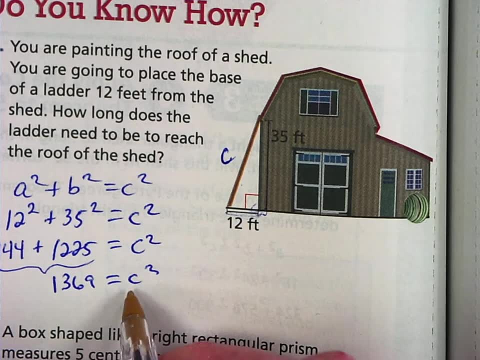 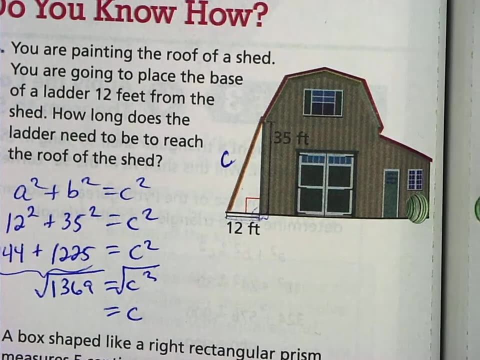 All right. so now, because these are on the same side, let's add these two together, So 144 plus 1,225 is 1,369.. And now I only want side C, not C, squared. So I'm going to square root both sides. So side C, the length of the ladder is 37.. 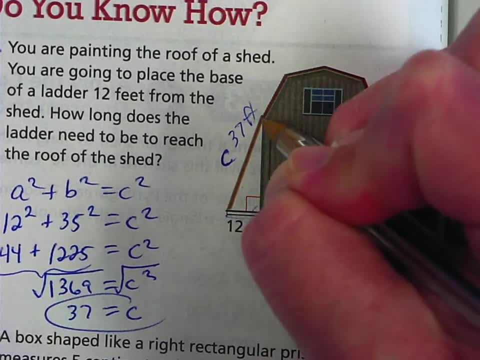 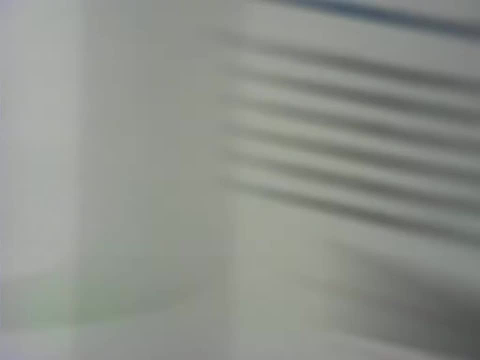 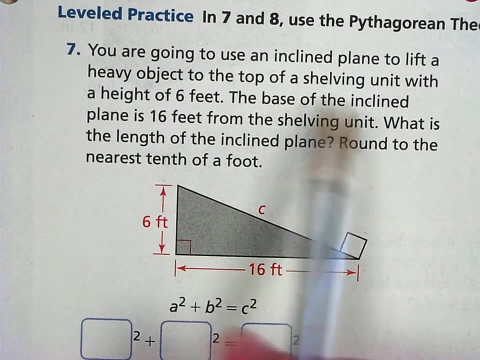 So that means that this needs to be 37 feet long in order to reach the top of the roof right there. Okay, let's take a look at another real-life problem. So you have this inch, So you have this incline plane right here and it says you're going to lift a heavy object to the very top of this shelf right here. 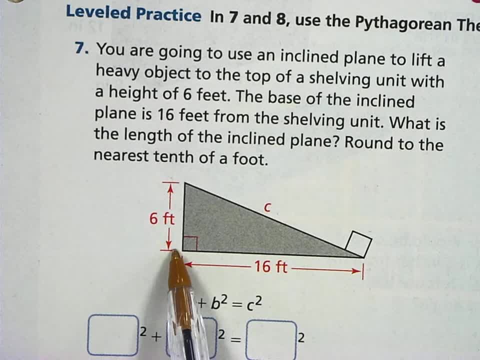 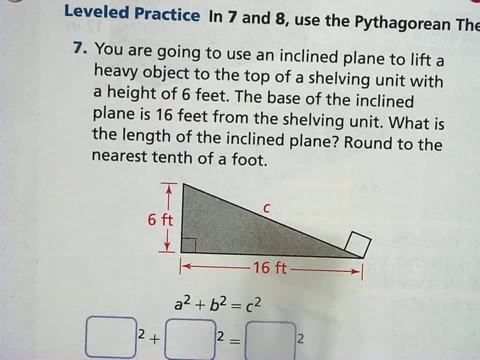 So it says the height of your plane is 6 feet, so that's labeled. The base of the incline plane is 16 feet from the unit, so it's 16 feet long And it says what's the length of the incline plane. 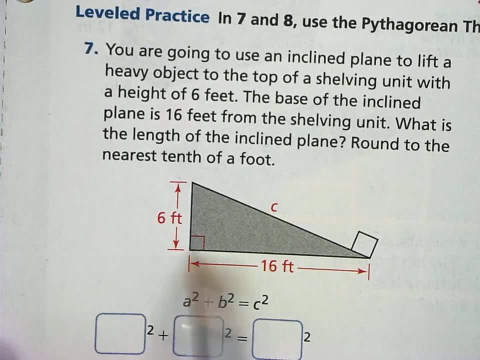 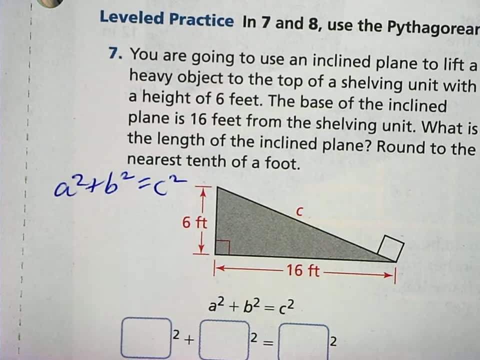 So we're missing the hypotenuse. So these are your legs. Again, they're connected to your right angle, your A and B. So I'm going to write A squared, That's B squared equals C squared, And we're going to figure out how long this has to be. 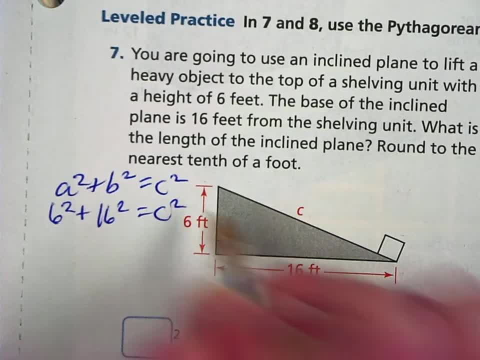 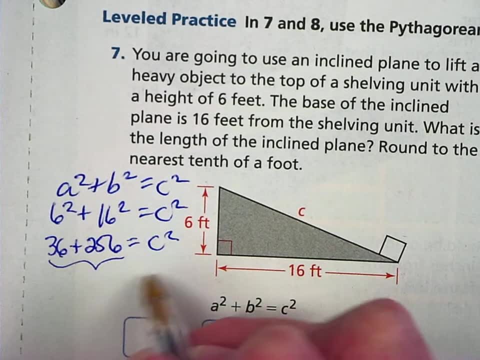 So 6 squared plus 16 squared equals C. squared 6 times 6 is 36.. 16 times 16 is 256.. Because these are on the same side, we're going to add these two together, So 292.. 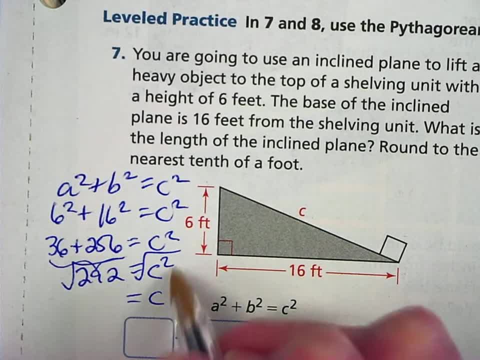 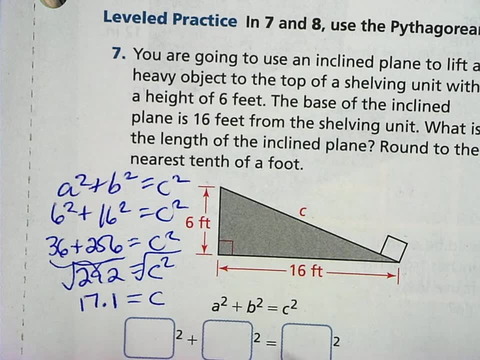 And then again I want to find the square root. So the square root of C squared is C And the square root of this. make sure you are rounding correctly. This says to the 10th place, 292 is not a perfect square. 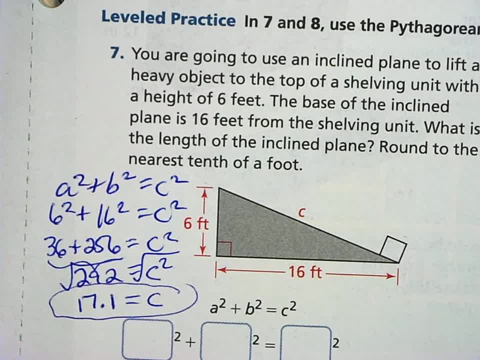 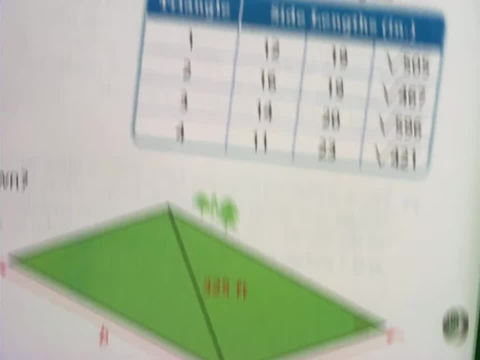 So you're going to get a decimal, But make sure you're rounding that decimal correctly. So the length of this has to be 17.1 feet. Okay, so let's do one more of those. So take a look at this rectangular plot of land. 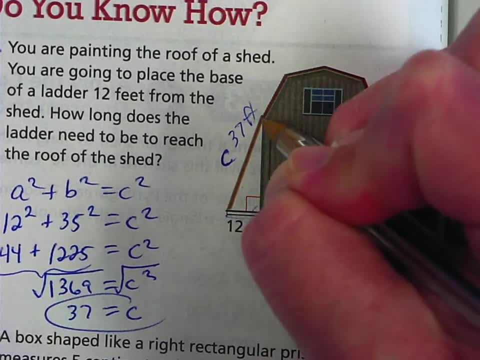 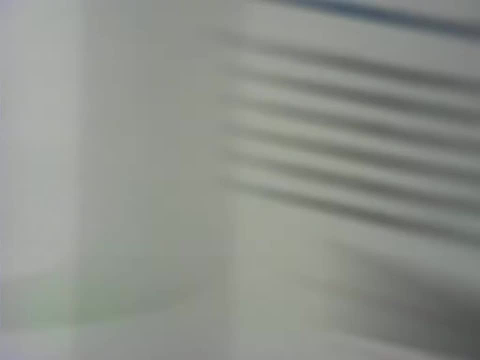 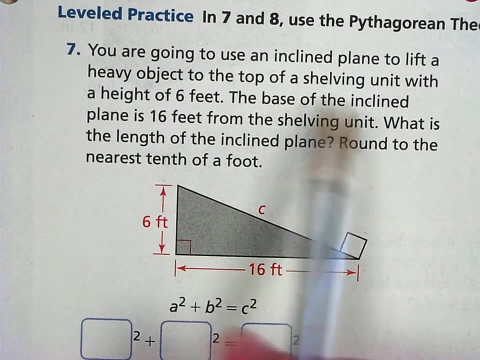 So that means that this needs to be 37 feet long in order to reach the top of the roof right there. Okay, let's take a look at another real-life problem. So you have this inch, So you have this incline plane right here and it says you're going to lift a heavy object to the very top of this shelf right here. 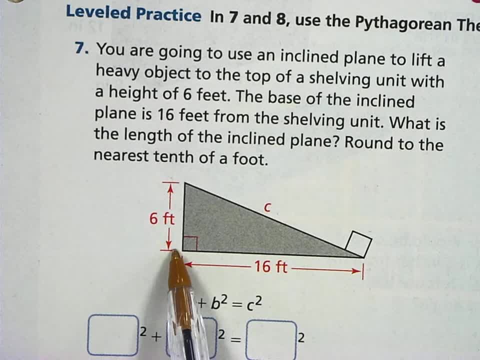 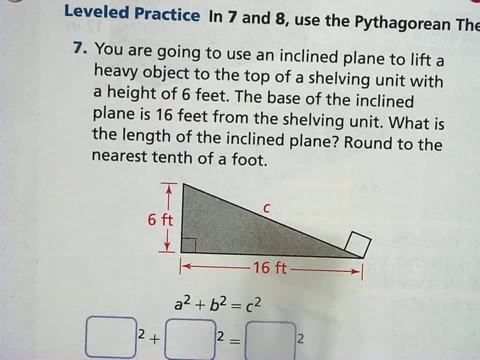 So it says the height of your plane is 6 feet, so that's labeled. The base of the incline plane is 16 feet from the unit, so it's 16 feet long And it says what's the length of the incline plane. 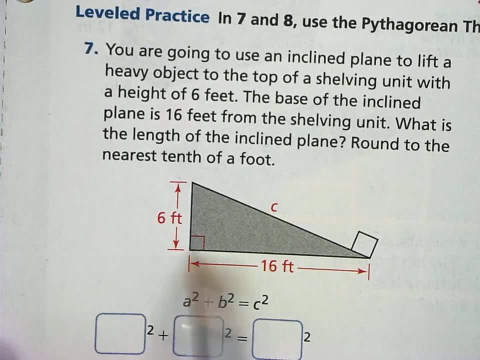 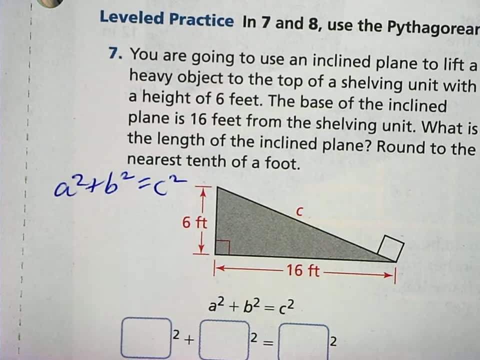 So we're missing the hypotenuse. So these are your legs. Again, they're connected to your right angle, your A and B. So I'm going to write A squared, That's B squared equals C squared, And we're going to figure out how long this has to be. 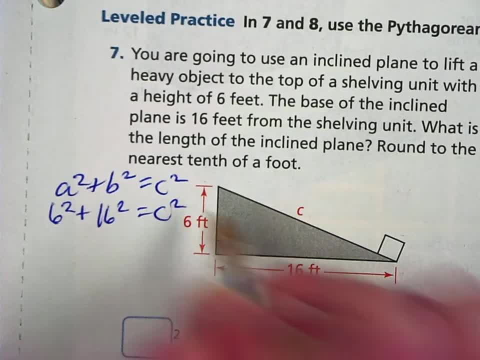 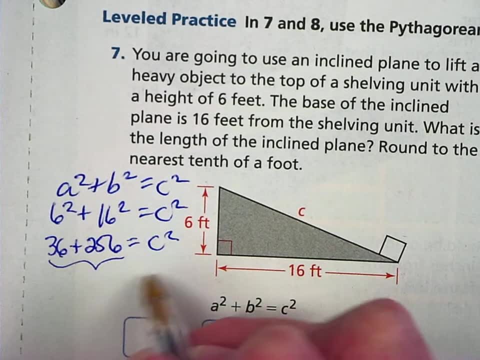 So 6 squared plus 16 squared equals C. squared 6 times 6 is 36.. 16 times 16 is 256.. Because these are on the same side, we're going to add these two together, So 292.. 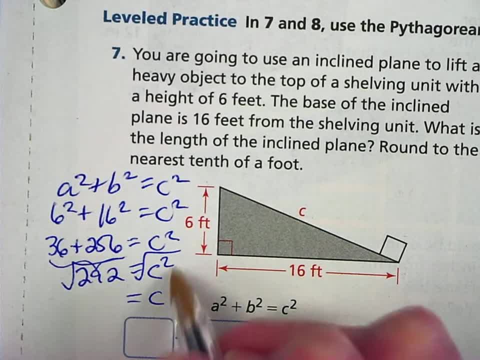 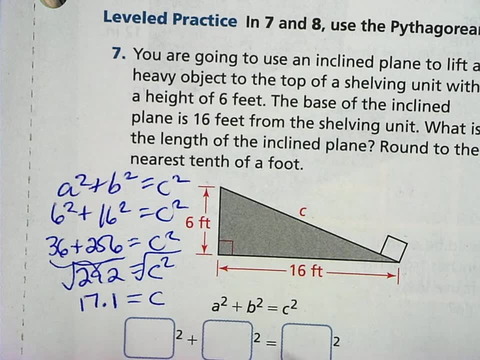 And then again I want to find the square root. So the square root of C squared is C And the square root of this. make sure you are rounding correctly. This says to the 10th place, 292 is not a perfect square. 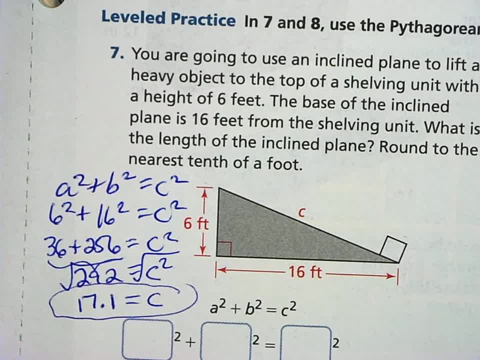 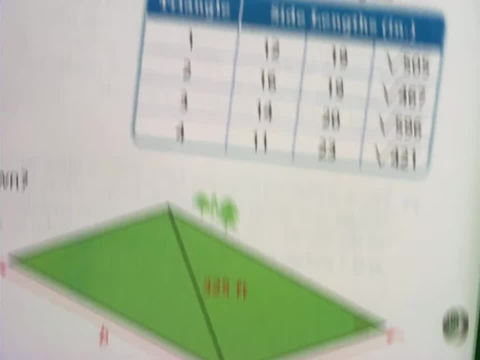 So you're going to get a decimal, But make sure you're rounding that decimal correctly. So the length of this has to be 17.1 feet. Okay, so let's do one more of those. So take a look at this rectangular plot of land. 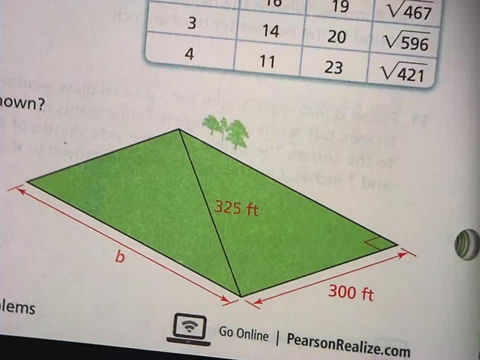 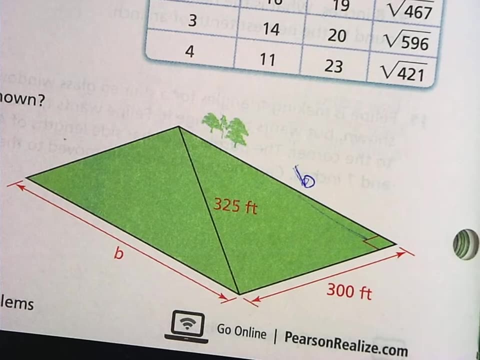 And it says: I want to find side B over here. Well, if this is just a rectangle, a flat rectangle, so this is also the same length as this. So it looks like you're missing one of your legs because the side directly opposite your right angle is your side C. 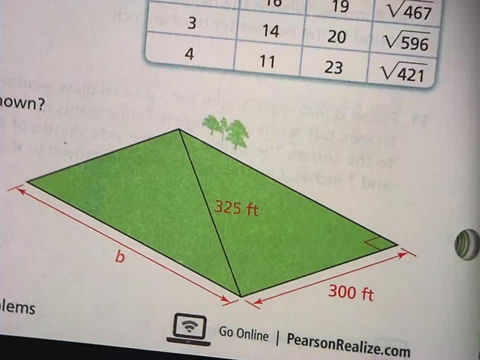 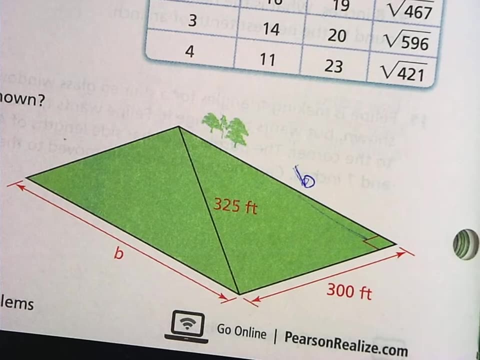 And it says: I want to find side B over here. Well, if this is just a rectangle, a flat rectangle, so this is also the same length as this. So it looks like you're missing one of your legs because the side directly opposite your right angle is your side C. 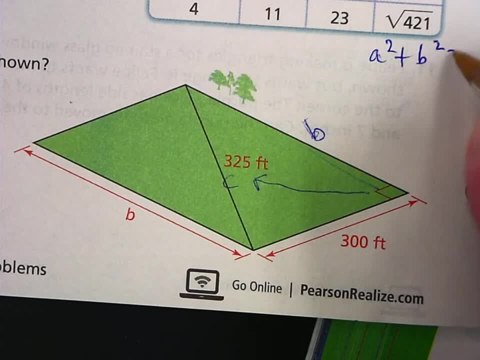 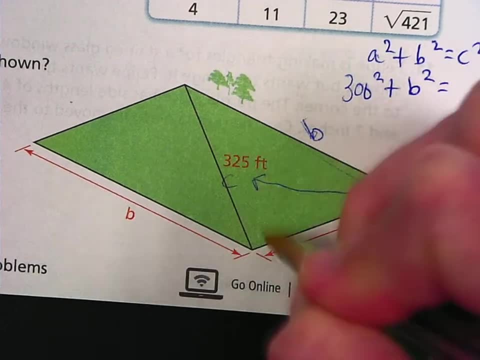 So let's try it: A squared plus B squared equals C squared. So this is my one leg. I have 300 squared And I'm missing the other leg, And then this is going to be my hypotenuse: 325 squared. 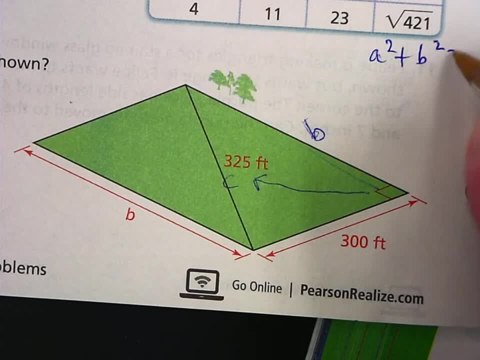 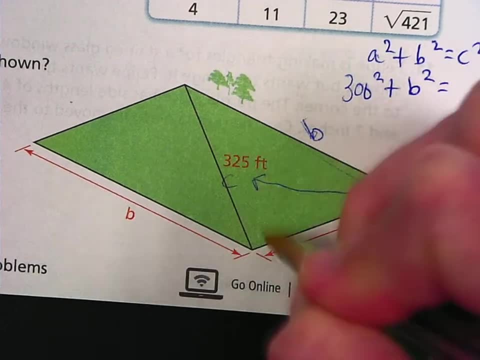 So let's try it: A squared plus B squared equals C squared. So this is my one leg. I have 300 squared And I'm missing the other leg, And then this is going to be my hypotenuse: 325 squared. 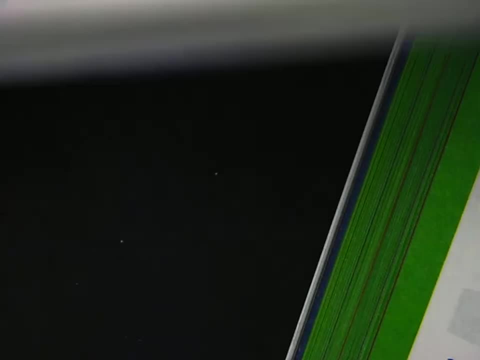 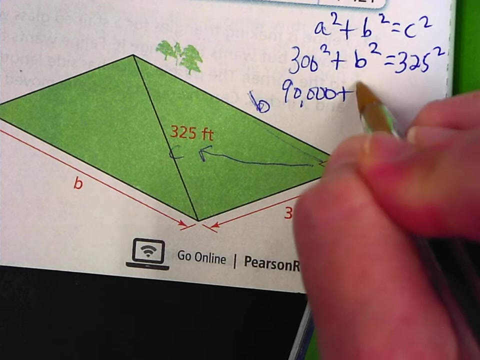 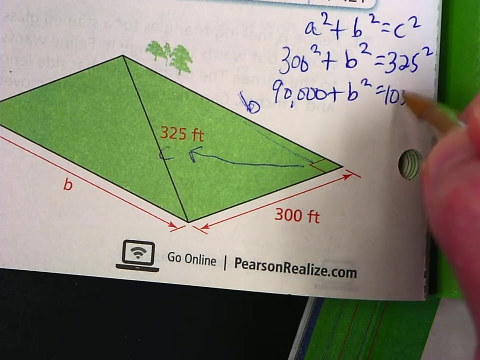 Okay, so let's solve that. So 300 times 300 is 90,000.. 325 times 325 is 145.. 145,625.. Now again, this is a good reminder, because these are on opposite sides. You have to subtract. 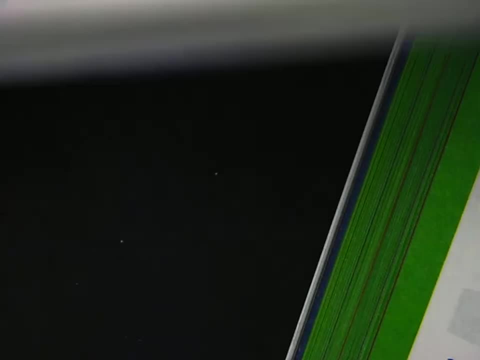 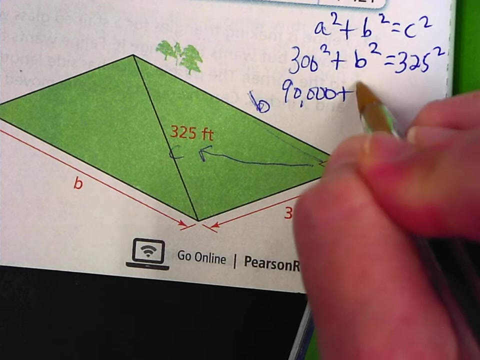 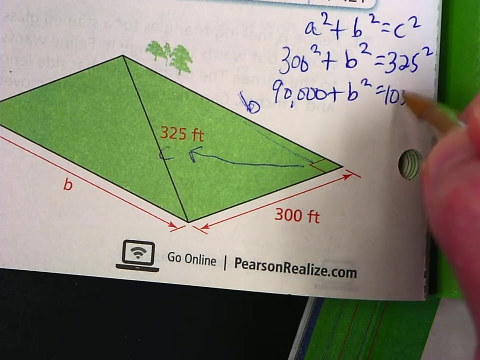 Okay, so let's solve that. So 300 times 300 is 90,000.. 325 times 325 is 145.. 145,625.. Now again, this is a good reminder, because these are on opposite sides. You have to subtract. 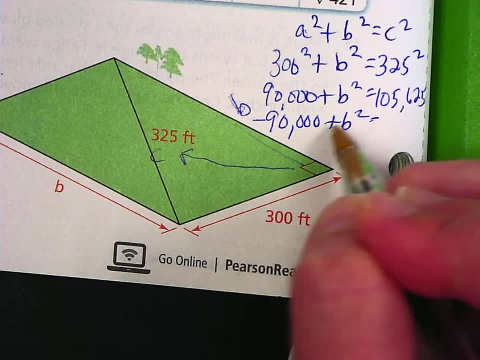 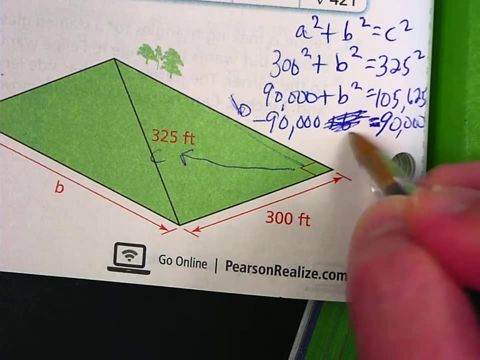 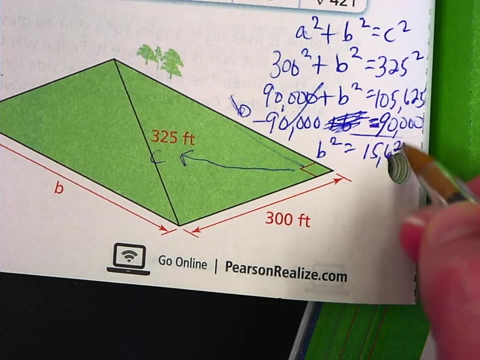 You have to get those two together on the same side. Actually, I don't need to bring that down yet. So we're going to subtract 90,000 from this side, So B squared is. so this takeaway, this is 15,625.. 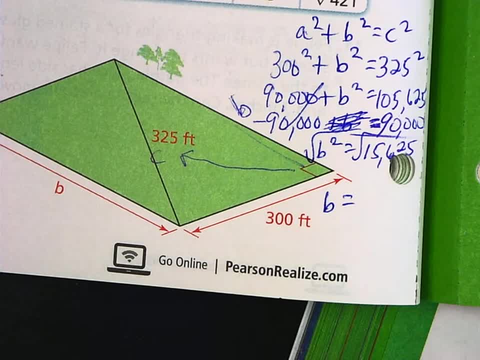 And then we're going to square root both sides. So the square root of B squared is B, And then the square root of 15,625 is 125.. And that is the length of this side of that plot of land. Okay, and I'm going to solve just one more for you that involve a square root. 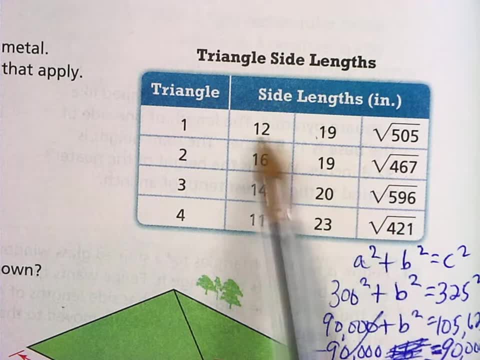 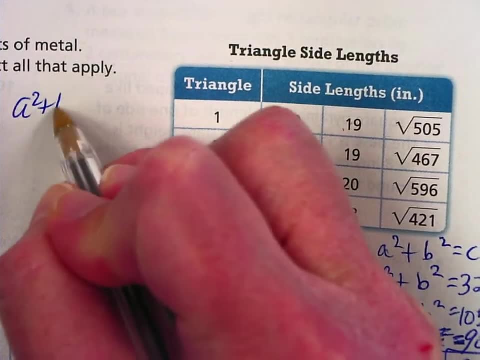 So let's see which one of these are right triangles. If we have three side lengths, this is the biggest number out of the three, So this has to be my C. So let's plug that in: A squared plus B squared equals C squared. 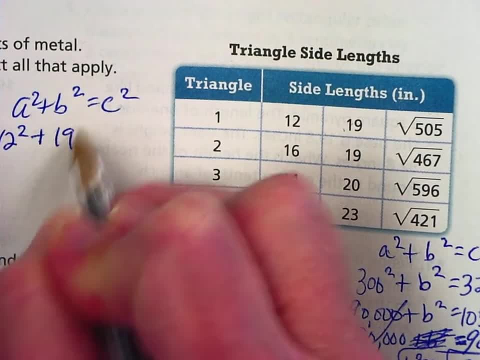 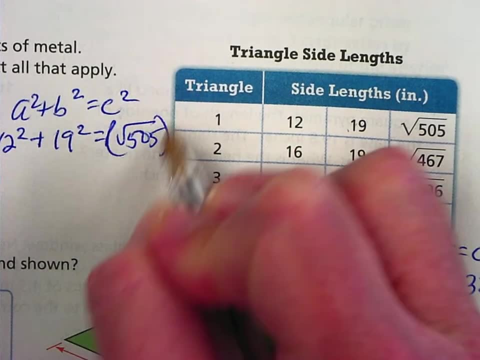 Okay, so let's make 12 squared plus 19 squared. Those are your A and B, your two legs, And then the square root of 505.. And, in parentheses, squared, we're going to square that. Okay, so 12 times 12 is 144.. 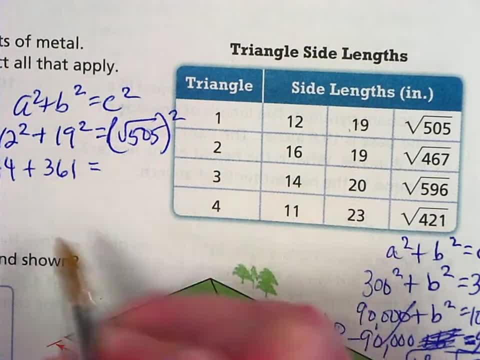 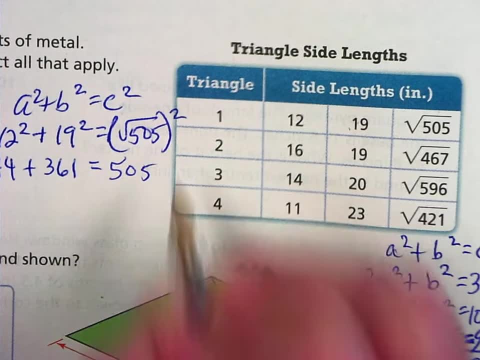 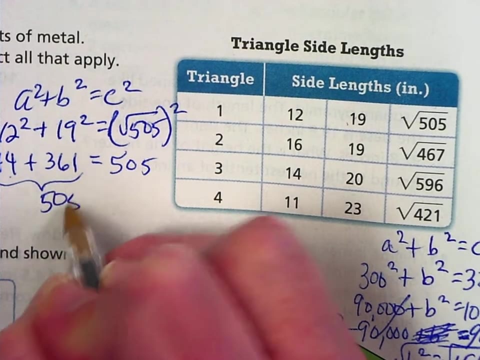 19 times 19 is 361.. And then the square root of 505 times the square root of 505 is 505.. So now let's add this side and see if it equals this side. So 144 plus 361 is 505.. 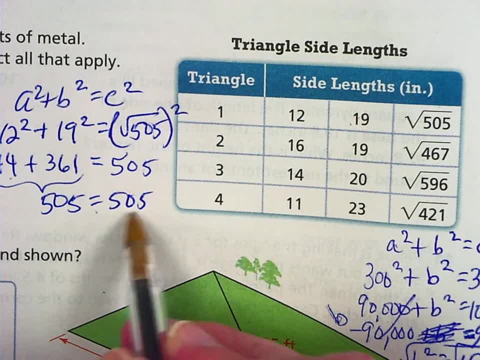 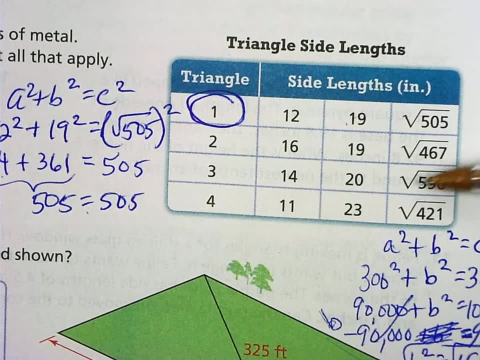 And since A squared plus B squared doesn't fit, it's going to be C squared. So if A squared plus B squared equals C squared, then triangle one is a right triangle, And you would go through and do the exact same thing with all of these. 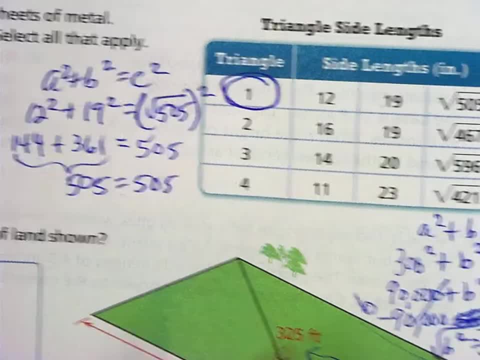 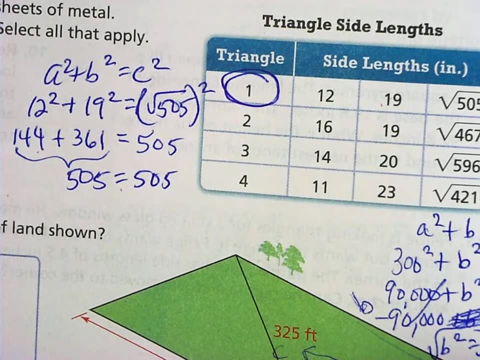 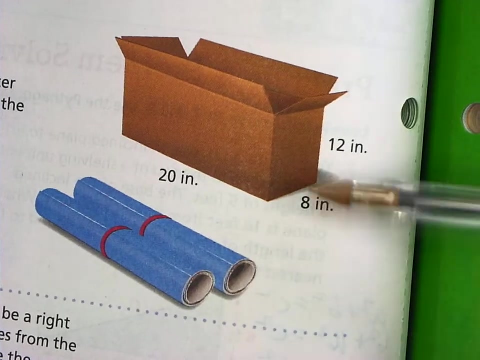 to see which ones were right triangles and which ones weren't. So now, folks, this is part one of this lesson, So I need you now to go in and watch part two. You've got to watch part two. I'm going to show you how to find the missing side lengths of a rectangular prism. 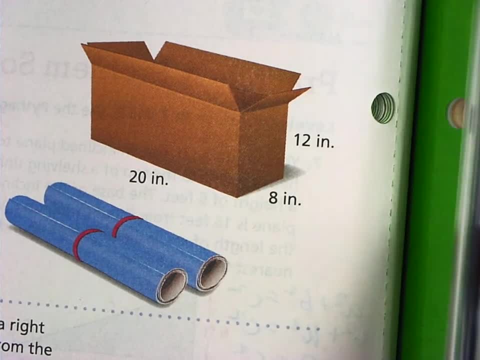 So that's a three-dimensional rectangle, kind of like a rectangle. It's like a shipping box right here. Go watch part two now. Thank you.